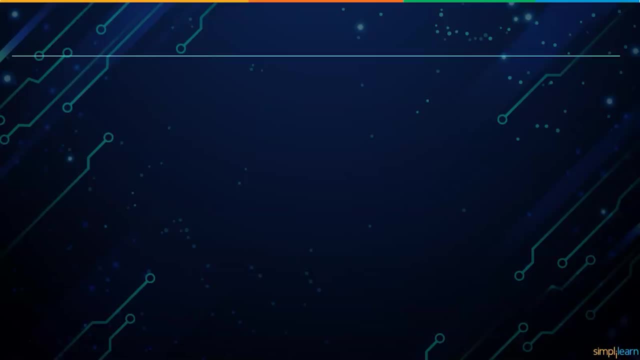 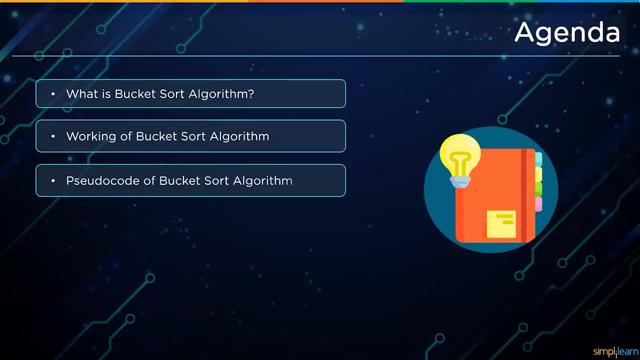 an update from Simply Learn Now. without further ado, let's get started with the agenda for today's discussion. At first, we will understand what exactly is a bucket sort algorithm. Next, we will understand the working principles of bucket sort algorithm, Followed by that. 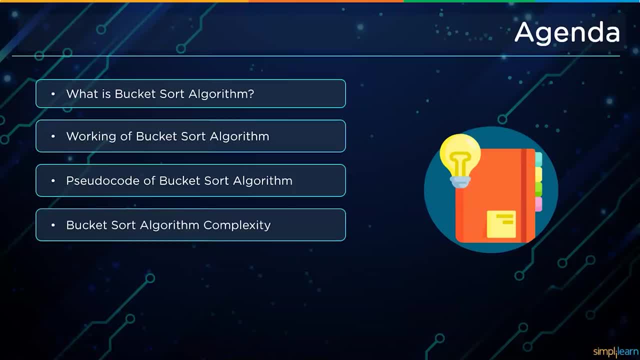 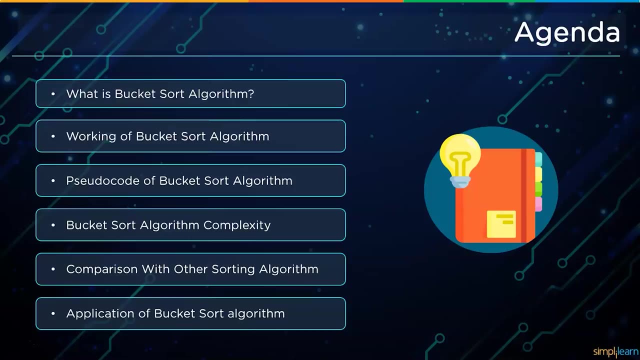 we will look at the pseudocode of bucket sort algorithm. Next we will understand the bucket sort algorithm's complexities. Then we will compare the bucket sort algorithm with other existing sorting algorithms. Finally, we will wind up the session by learning the various applications of bucket sort algorithms. So I hope I made myself clear with the agenda. 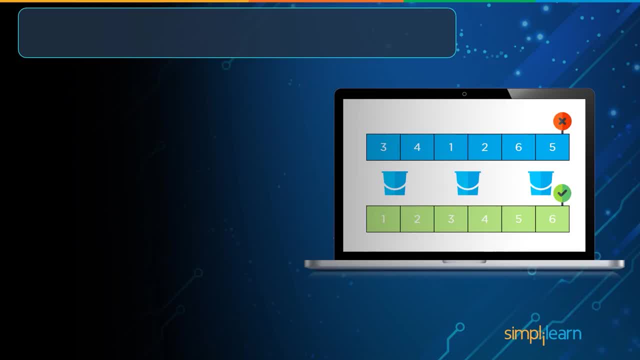 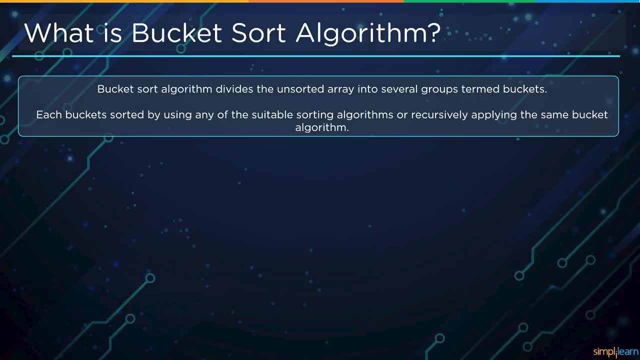 Now let's get started with our first concept, that is, what exactly is a bucket sort algorithm? So the bucket sort algorithm divides the unsorted array into several groups known as buckets. So each bucket is sorted using any suitable sorting algorithm or recursively. 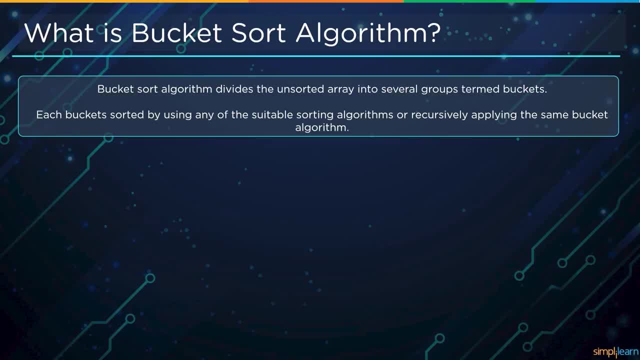 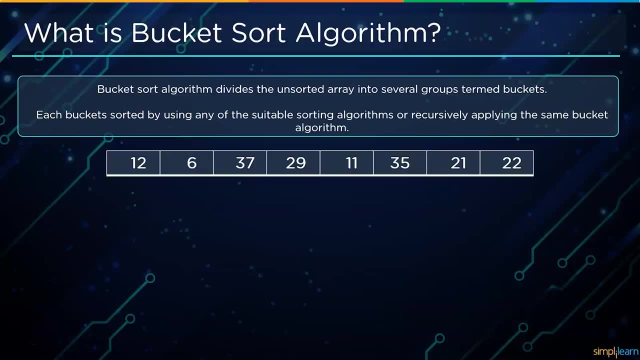 applying the same bucket sort algorithm. I know it, it's a little complicated, So let's go through an example of a bucket sort algorithm. Let's look at our first example. On my screen we have an example of an array consisting: 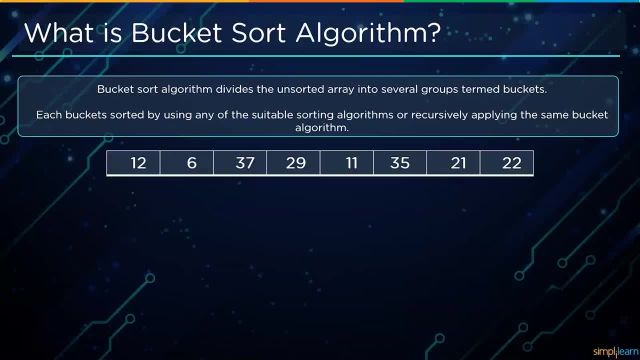 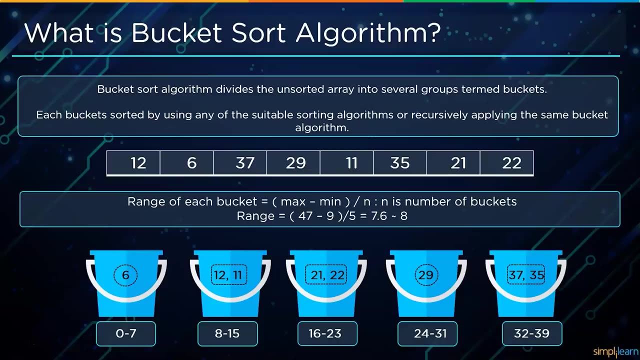 of a bunch of numerical elements, that is, 25,, 12,, Eliad, 33,, 17,, 36 and 12.. Now let's see the other bucket sort algorithms. First we are going to look at multiple buckets with different ranges. Every gene of the first string has different ranges from 6, g, 3,. 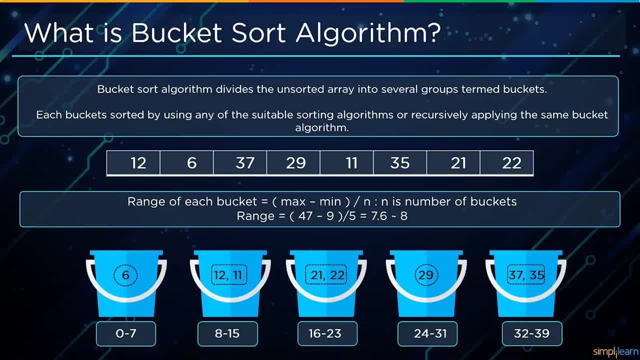 4,, 5, 6……… okay, I need a bracket: 23, 24 to 31 and finally the last bucket with range 32 to 39. so 6 will be stored in the first bucket, followed by that 11 and 12 will be stored in the second bucket, followed by that we have 21. 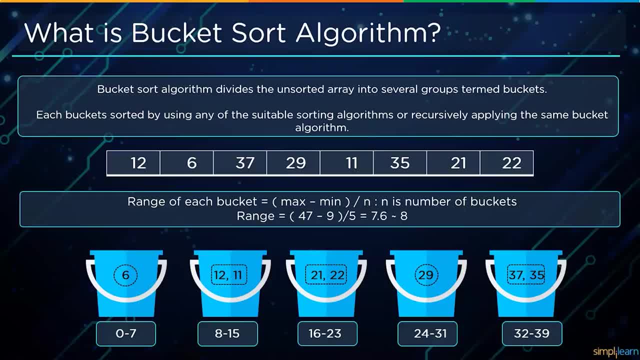 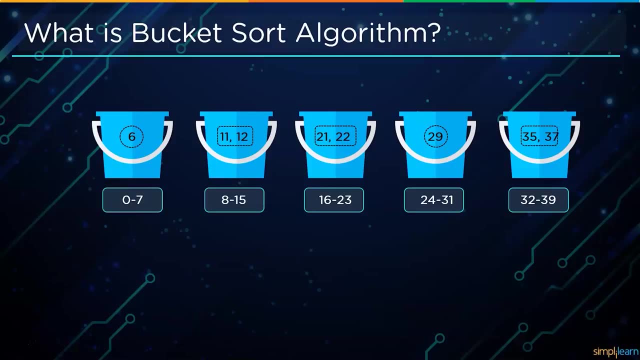 and 22 stored in the third bucket, followed by that we have 29 in the fourth bucket and finally the last two elements, which are 37 and 35, stored in the last bucket. in the next stage, all the elements are sorted according to an order that might be ascending. 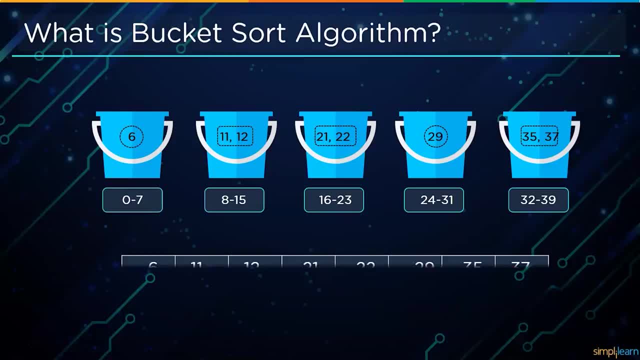 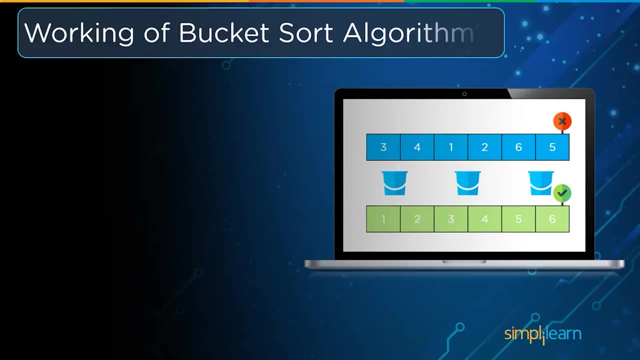 or descending. in our case, we have the ascending order, so the final result will be 6, 11, 12, 21, 22, 29, 35 and 37. so this is how the bucket sort algorithm works in real time. now the next topic, that is. 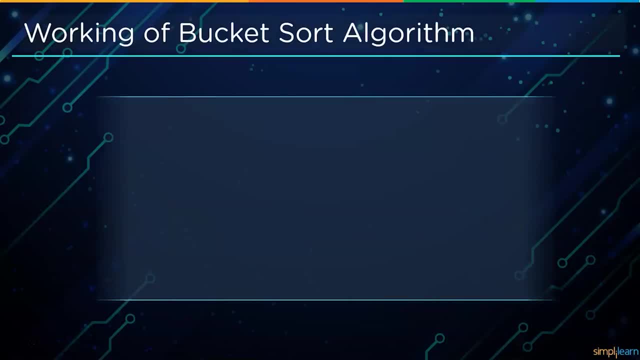 working off a bucket sort algorithm in a detailed way. so now we don't have to worry about the order of the elements, we just have to think about the order of the elements. so now we don't have to worry about the order of the elements, we just have to think about the order of the elements. 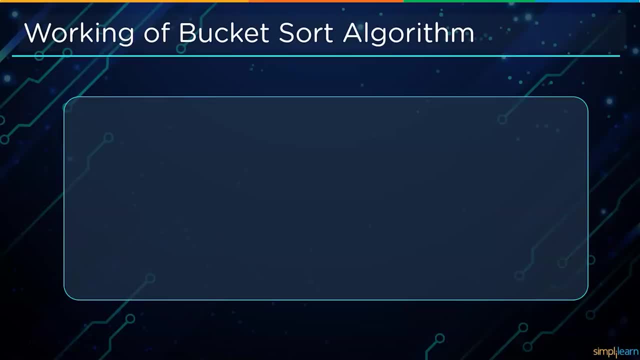 know the briefing of a bucket sort algorithm. now let's learn the working of bucket sort algorithm in depth. suppose we have an array consisting of decimal values or floating values as the input. so the first element is 0.47, next we have 0.39, 0.23, 0.55, 0.29, 0.41, 0.59 and finally 0.31. then we will. 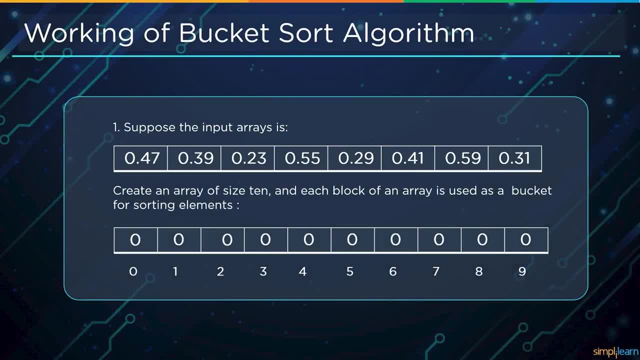 create an array of size 0.39 and finally 0.31. then we will create an array of size 0.39 and finally 0.31. then we will create an array of size 0.39 and finally 0.31. then we will create an array of size 10 and store 0 in each block and each block. 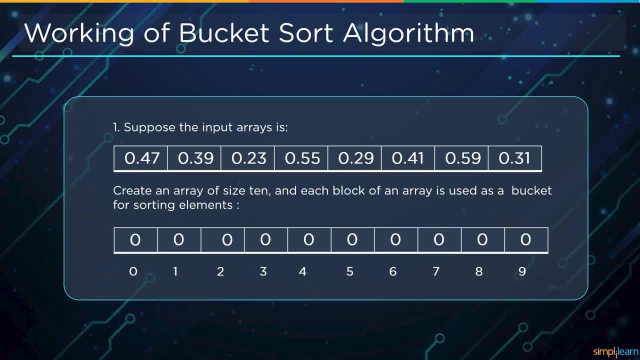 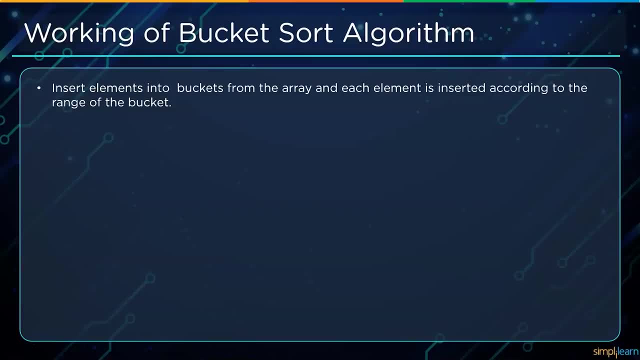 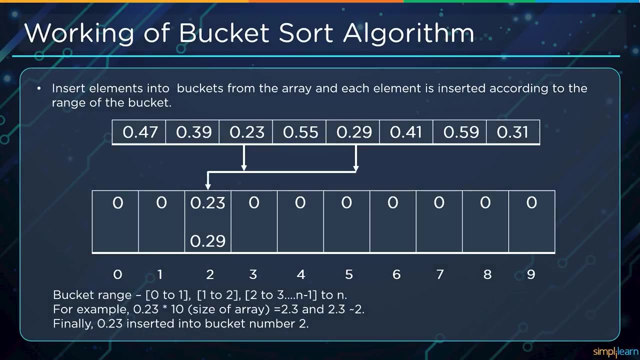 of an array is used as a bucket for sorting the elements. next we have step 2: insert the elements into buckets from the array and all elements are inserted as per the range of the bucket buckets, ranging from 0 to 1, 1 to 2, 2 to 3, up to n minus 1 to n. here n is the number of elements in. 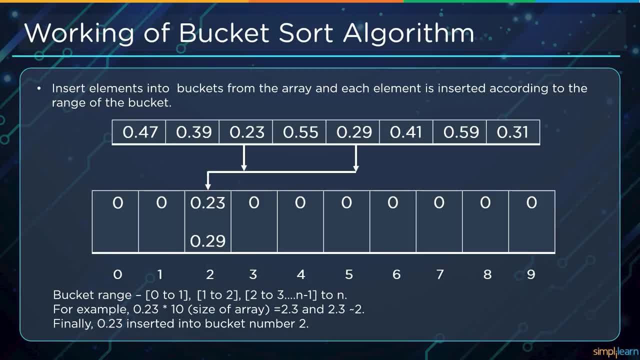 an array, so n is the number of elements in an array, so n is the number of elements in an array. so, for our example, 0.23 will be multiplied by 10, which is the size of an array, and that gives us 2.3. 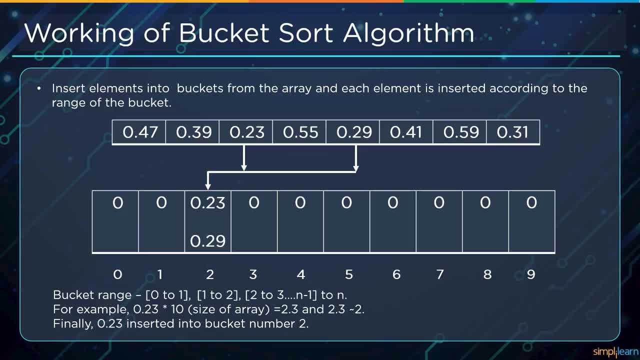 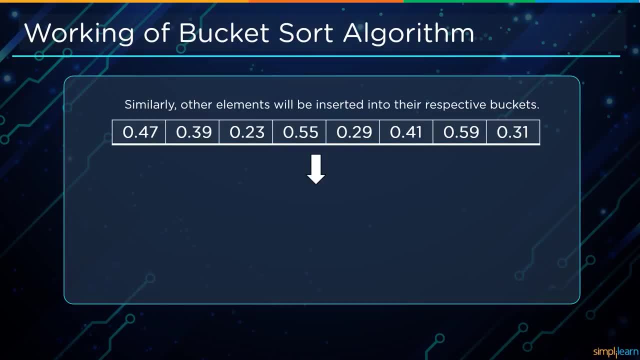 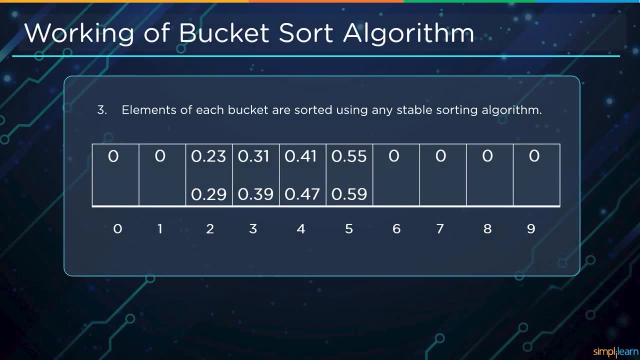 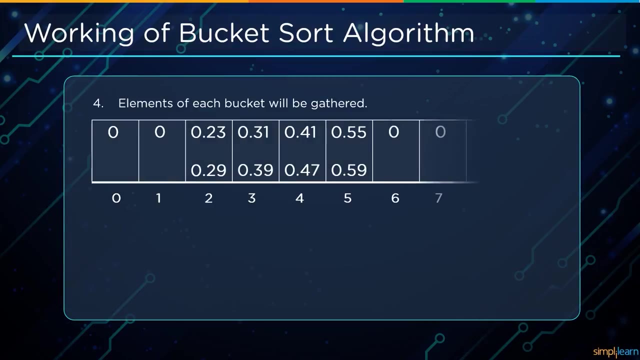 approximately equal to 2. so finally, we will insert 0.23 into the bucket number 2. in exact, we will insert other elements into other respective buckets. followed by that, we have step 3- elements of each bucket are sorted using the stable sorting algorithms- and finally, the step 4. in step 4, all the sorted elements of each bucket will be gathered. 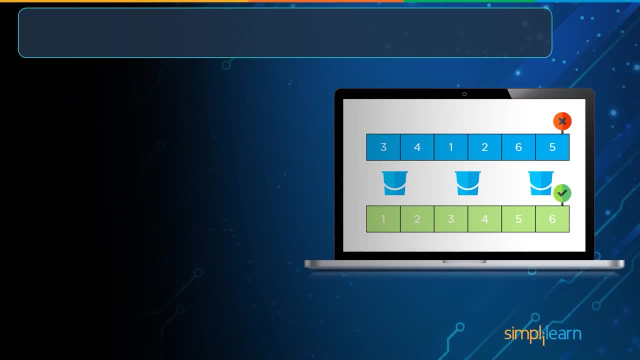 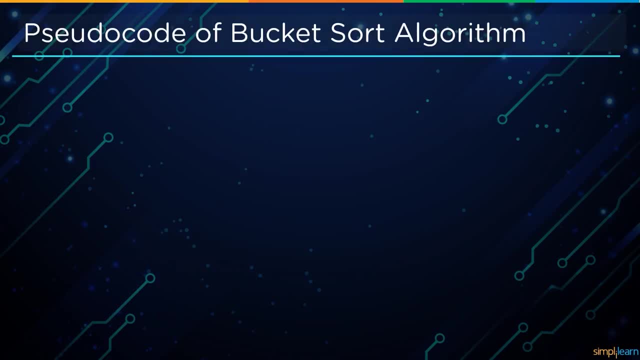 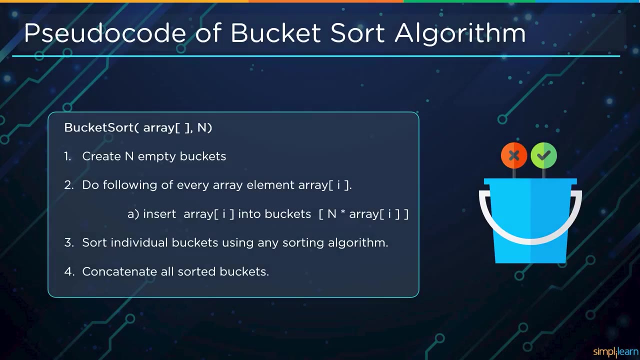 and represented in the form of an array. as pseudocode is an informal programming description that does not require any strict programming language syntax. similarly, we will understand it effortlessly. so in the pseudocode, first we will create n empty buckets. next we will insert all the array elements into buckets by multiplying the size of the bucket by. 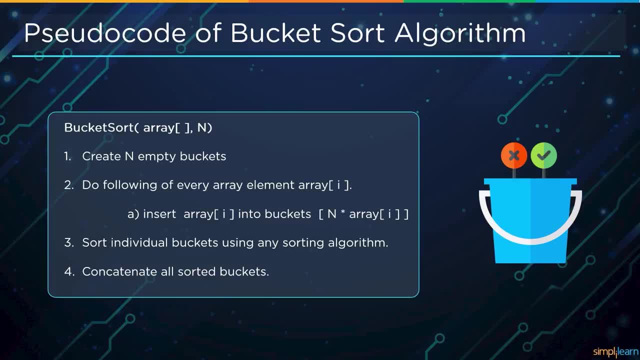 their size left and right. we keep doing that to create a bar space in each building, so we get answers quite easily that way. we have to keep doing this for every array element, as we understood this in working of the bucket sort algorithm. after that we have to sort individual. 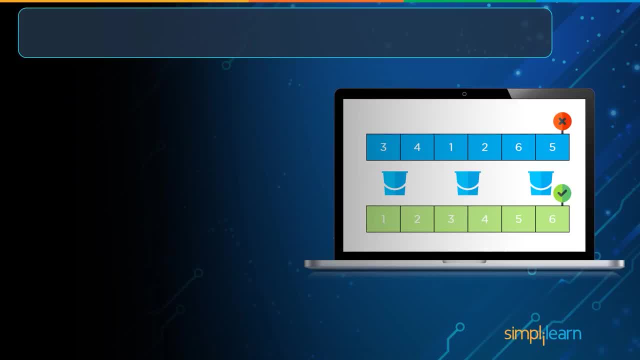 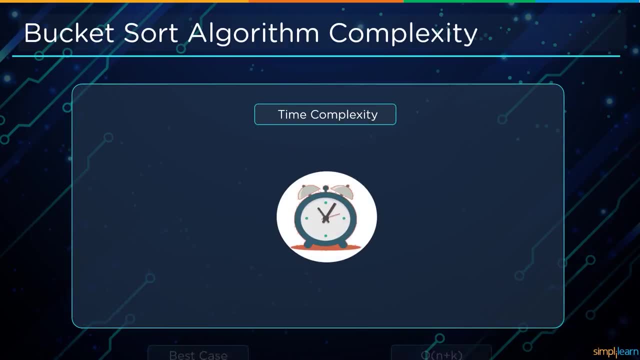 buckets using insertion sort and finally, we will concatenate all the sorted buckets. next, we will learn about the complexities of bucket sort algorithm. first we will see about time complexity. so, talking about the time complexity and ihr systems, their time types, you can usually have the best ones and the least types you can generate. time complexity levels are always comparable. 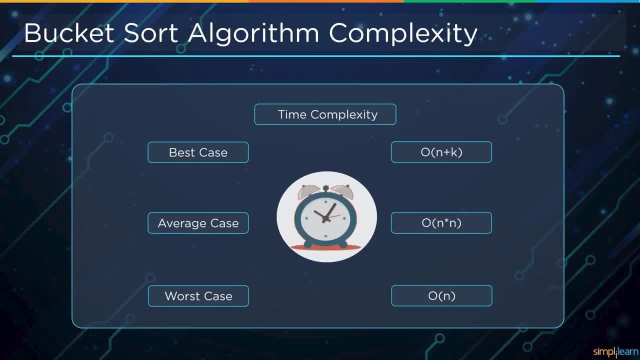 So first we have the best case, so that the best case is O. next we have the average case, that is O, and finally we have the worst case, that is O. Here N is the total number of elements to be sorted and K is the number of buckets. 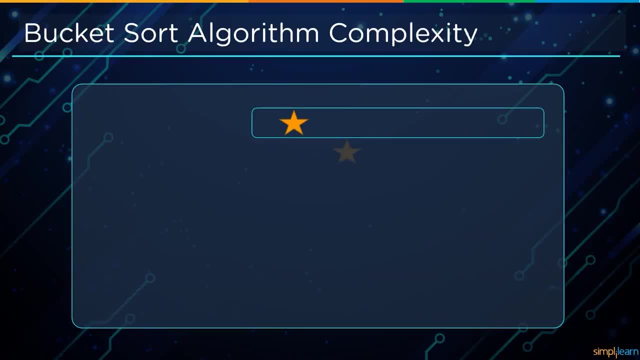 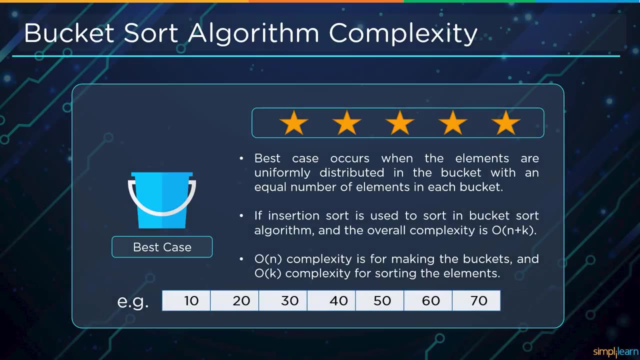 So let us understand all the three cases one by one. So first we have the best case. so the best case occurs when all the elements are uniformly distributed in the bucket, with an equal number of elements in each bucket. If insertion sort is used to sort the bucket sort algorithm, then overall time complexity. 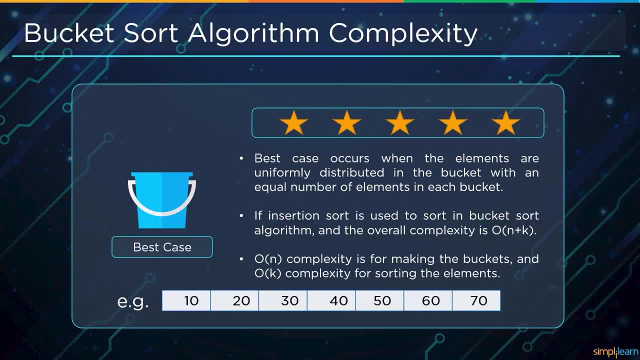 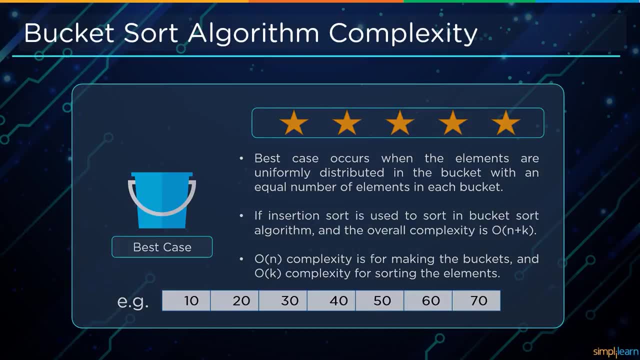 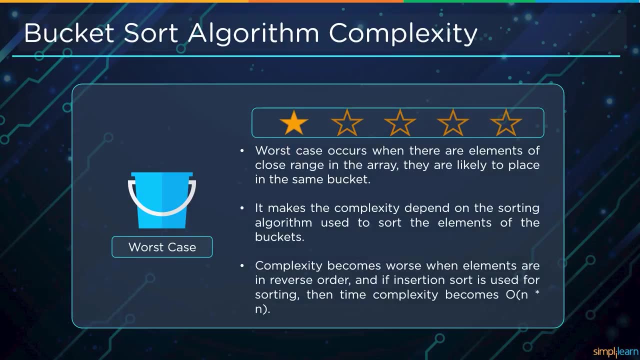 is O. O complexity is for making the buckets and O complexity is for sorting all the elements. After understanding the best case, now we will see how the worst case occurs in the bucket sort algorithm. The worst case occurs when there are elements of close range in the array. 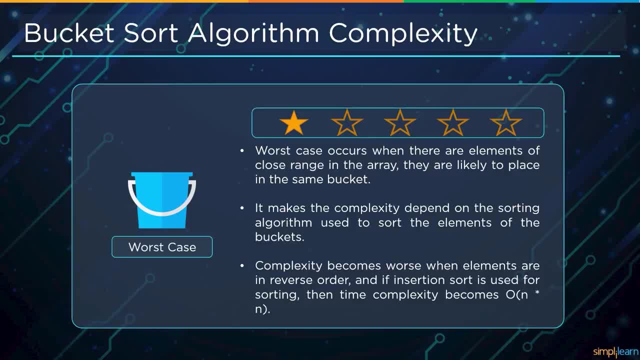 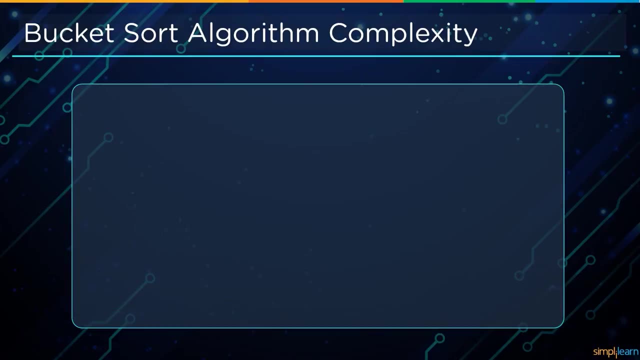 They are likely to be placed in the same bucket. It makes the complexity depend on the sorting algorithm used to sort the elements of the buckets. Complexity becomes worse when all the elements are in reverse order and if insertion sort is used for sorting, then time complexity becomes O. 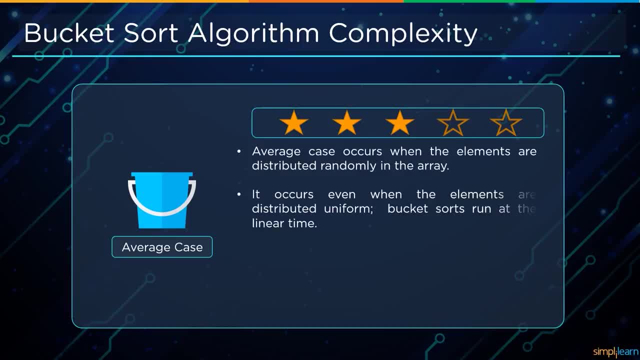 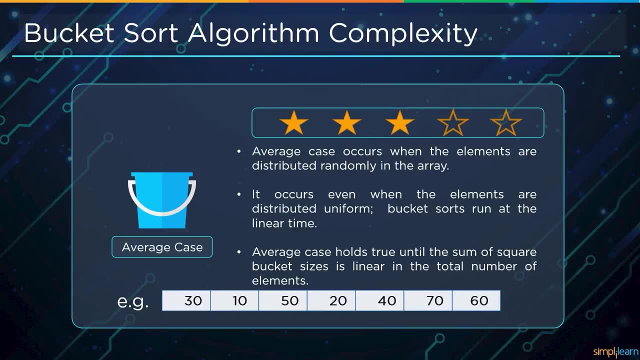 And lastly, we will learn how the average case occurs in a bucket sort algorithm. The average case occurs when the elements are randomly distributed in the array. It occurs even when the elements are in reverse order. So the worst case occurs when the elements are randomly distributed in the array. 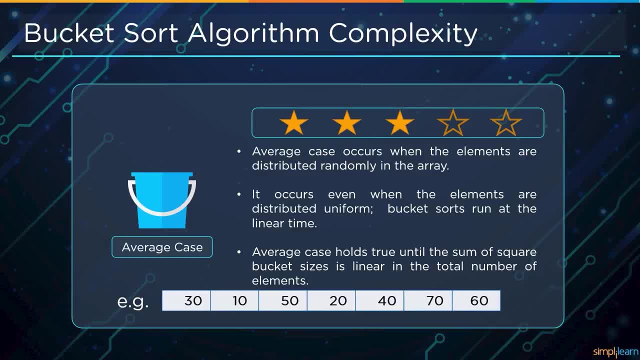 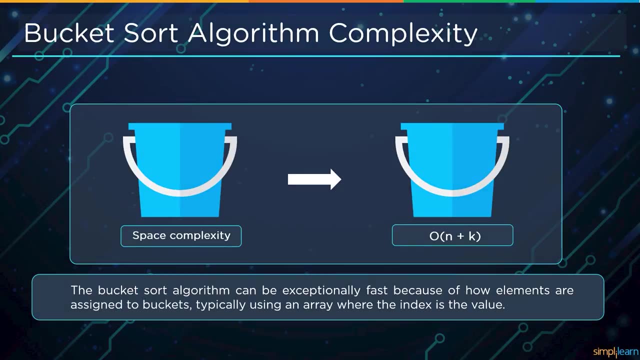 The bucket sorts run at the linear time. The average case holds true until the sum of bucket sort sizes is linear and in the total number of elements. Next we will see about the space complexity. So the space complexity of all the bucket sort algorithms is O. 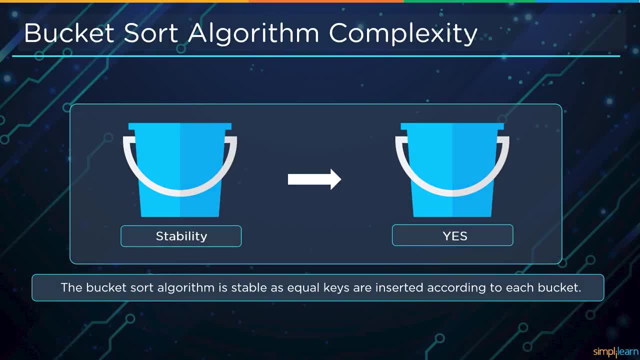 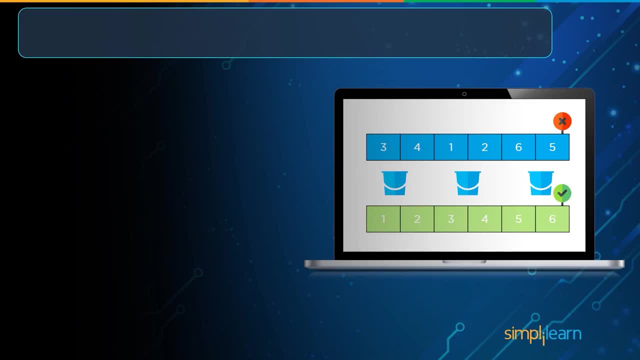 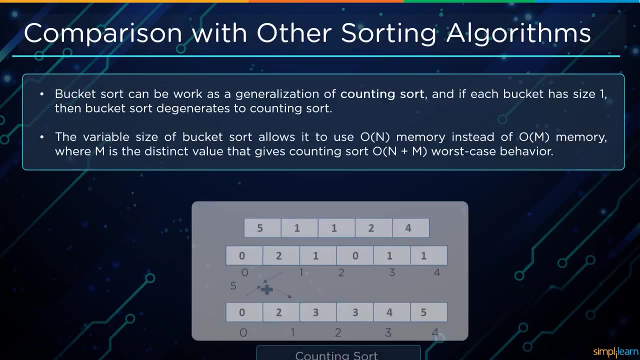 Lastly, we have stability. So talking about stability, so yes, the bucket sort algorithm is stable. After understanding the complexity of the bucket sort algorithm, now we will compare the bucket sort algorithm with other algorithms. So first we will compare the counting sort algorithm. 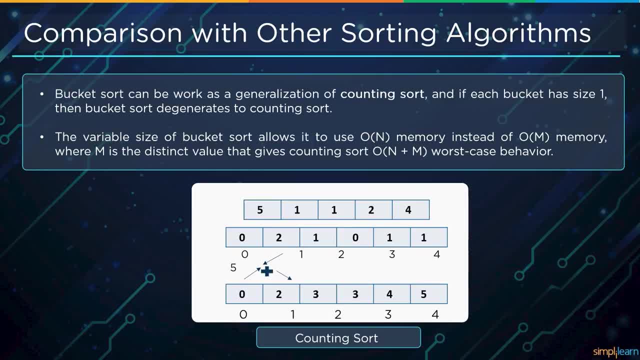 Bucket sort can be worked as a generalization of counting sort algorithm And if each bucket has size one, then the bucket sort degenerates to counting zero. The variable size of the bucket sort algorithm allows it to use O. We can also see that the countless countings are nationwide. 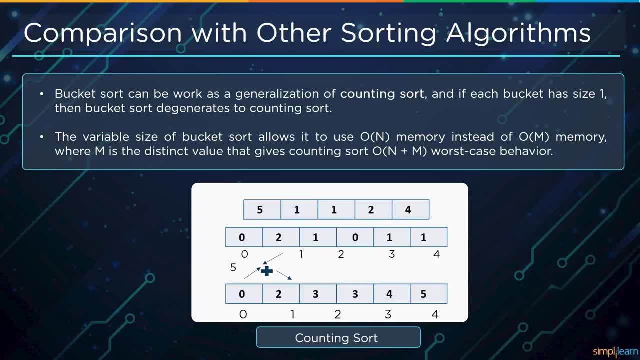 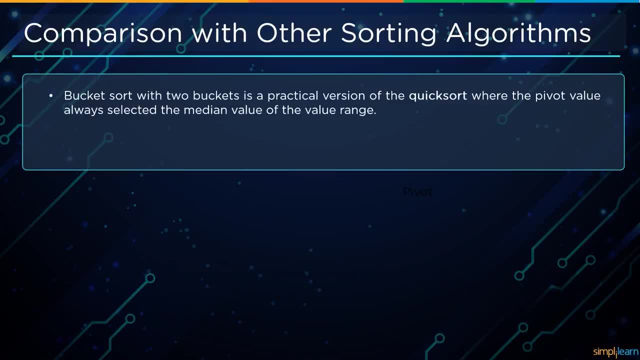 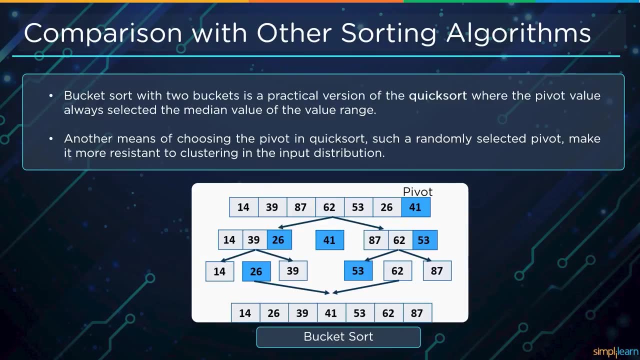 So if each number of buckets has size one, then the bucket sort degenerates to counting instead of O, where M stands for the distinct value that gives counting sort O worst case behavior. Next we will compare the bucket sort algorithm with quicksort. Bucket sort with two buckets is a practical version. 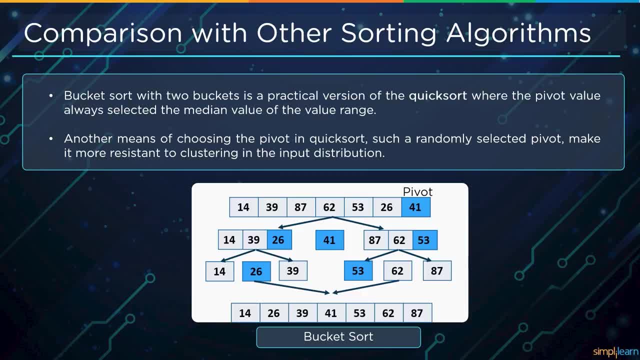 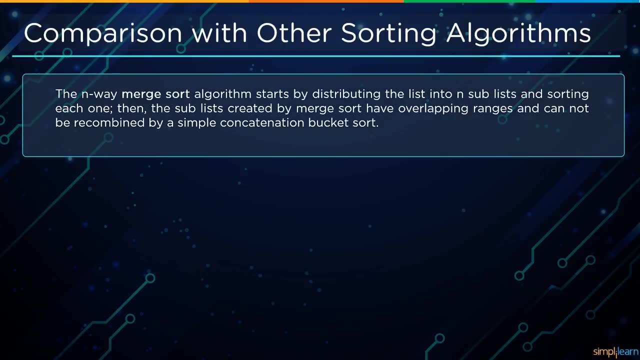 of the quicksort, where the pivot value always selects the median value of the value range. Another meaning of choosing the pivot in quicksort, such as a randomly selected pivot, makes it more resistant to clustering it in the input distribution. After that we have the merge sort, The n-way merge sort algorithm. 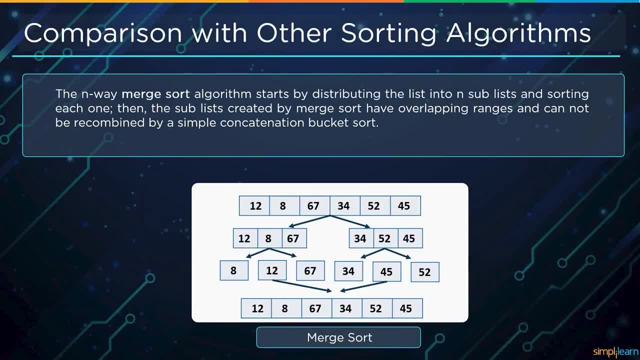 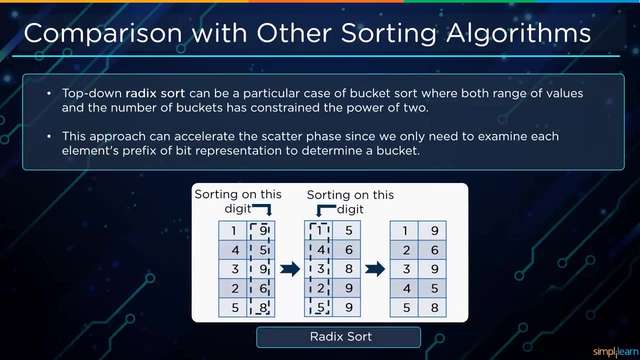 starts by distributing the list into n sub lists and sorting each one. Then the sub lists created by merge sort have overlapping ranges and cannot be recombined by a simple concatenation bucket sort. Lastly, we have one more sorting algorithm, that is radix sort. for comparison. 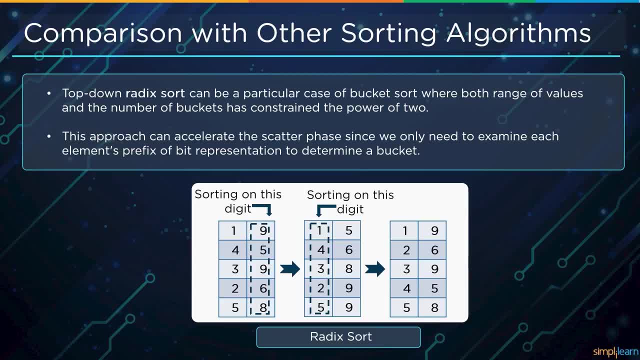 Top-down radix sort can be a particular case of bucket sort where both range of values and the number of buckets has contained the power of 2.. This approach can accelerate the scatter phase, since we only need to examine each elements prefix of bit representation to determine a bucket. At last we have one. 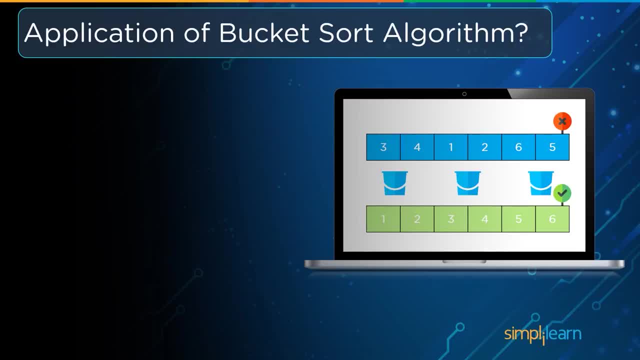 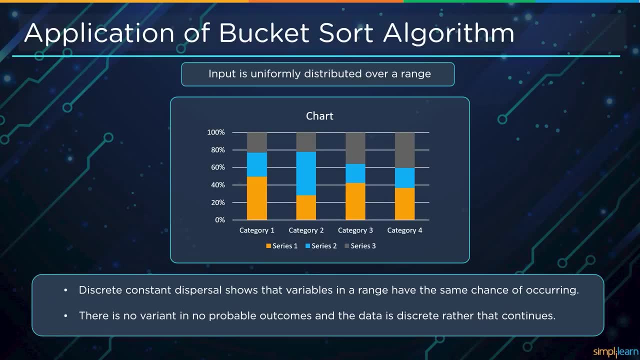 more topic to learn, that is, the applications of bucket sort algorithm. The bucket sort algorithm consists of two main applications. First, by using bucket sort algorithm, input is uniformly distributed on the range And second, by using bucket sort algorithm, there are floating point. 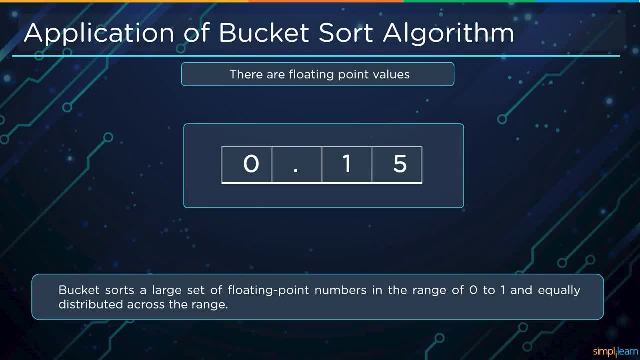 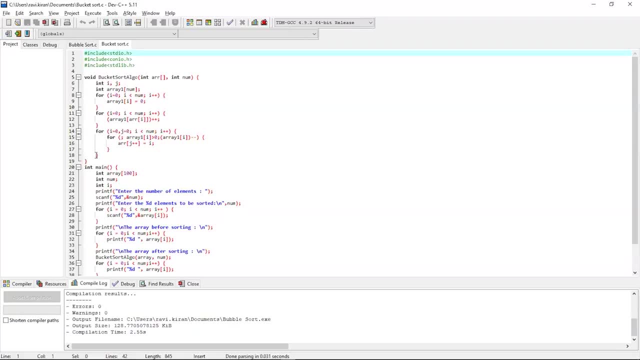 values. Now let us go through a practical demonstration of bucket sort algorithm. Now on my screen we have an example for bucket sort algorithm. So we will begin with the header files, followed by that we will define a function, namely bucket sort algorithm. This particular function is to implement a bucket. 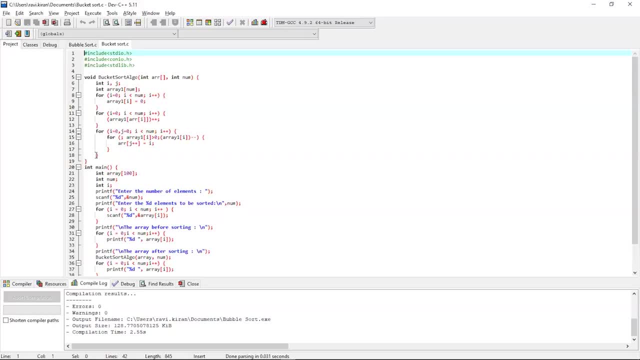 sort algorithm. In the function's argument there will be an array, namely arr, and a variable, num, which will store the number of elements in an array. After that, we will define two counter variables, which are i and j, and declare one more array, namely array1, with the same. 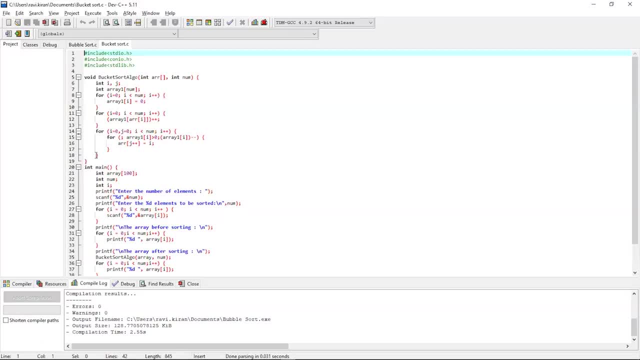 size of an arr array. So this particular second array will be used for displaying all the elements in the array1.. We will have a for loop which will run from index 0 to the entire size of an array, and for this array we will use 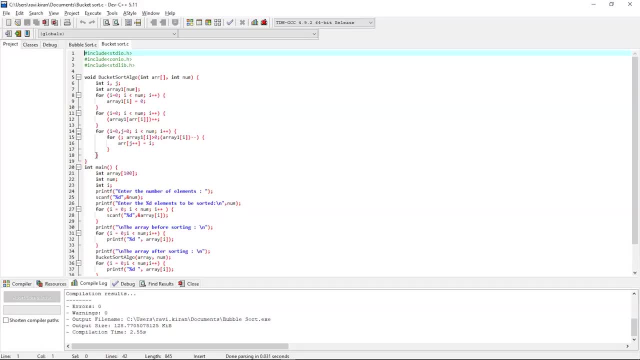 the variable i as the counter variable. We will have another for loop to print all the repeated numbers with frequency in an array. We will run another for loop from index 0 to the last element of both the arrays and elements of array, and array1 will assigned. 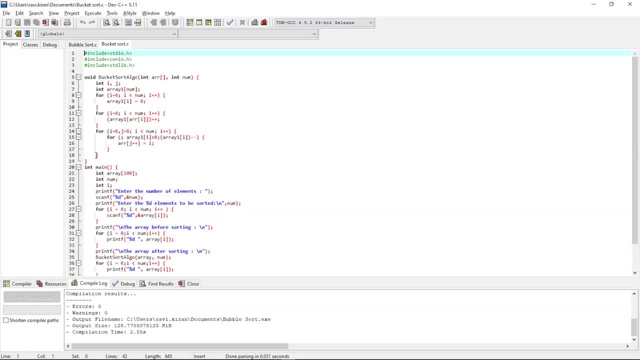 to arr array. Now we will execute from both the loops and now we will enter the into the main function where we will declare an array, namely array with the size of 100 and two variables which are num and I. next we will ask the user to: 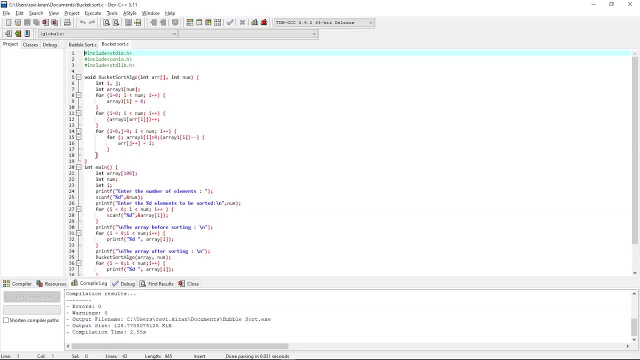 enter several elements of an array using printf function and now the user will enter number of elements and we will scan that using the scanner function. now we will ask the user to enter the elements of an array using printf function and the entered elements will be scanned using the scanner function. 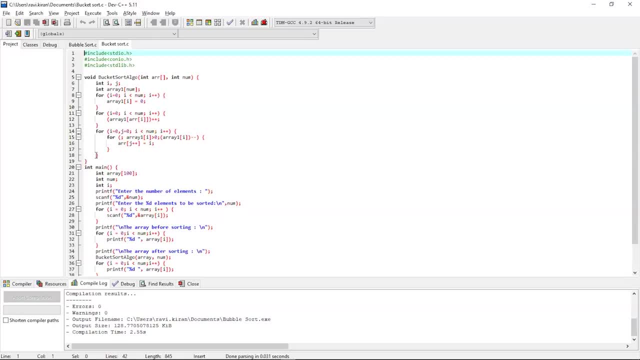 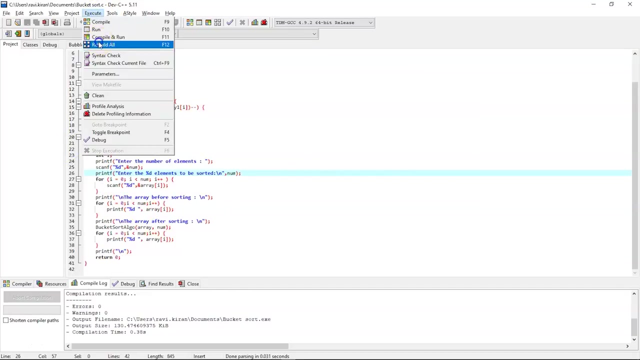 and next we will print a before sorting and an array after sorting, using for loops by calling the packet sort algo function and in this function we will pass the name of an array- that is an array- and the size of an array- that is num. now let us try to execute this program and see the output.